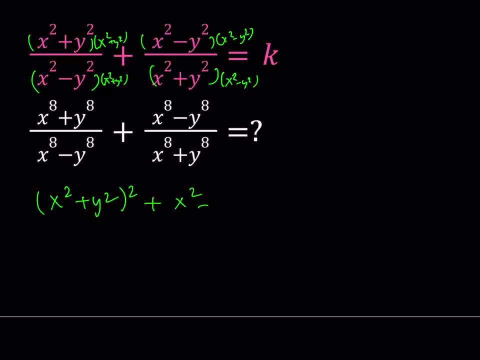 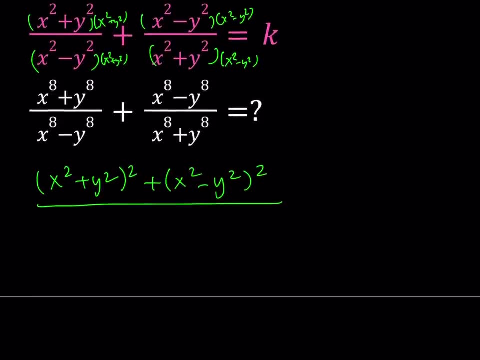 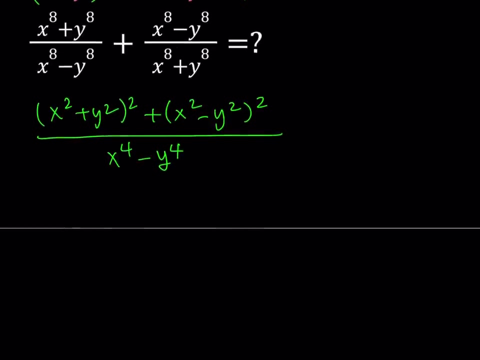 quantity squared plus x squared minus y squared quantity squared And that is going to be divided by these two expressions, the product, and that's going to be difference of two squares. So I can write it as x to the fourth minus y to the fourth. Now, if you expand this expression, you probably 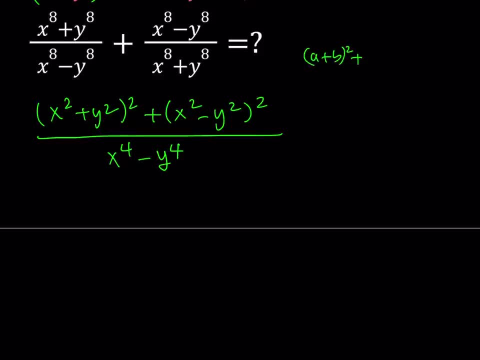 know that if you add a plus b squared and a plus b squared, you're going to get x to the fourth minus y to the fourth, And if you add a minus b squared, that should always equal to two times the quantity a squared plus b squared, because the two ab in the middle cancels out. So we are going to be getting from. 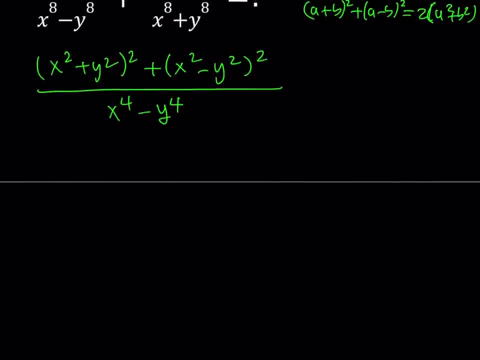 here the expression something like this: we're going to get x to the fourth power plus y to the fourth power, but just twice. And at the bottom we're going to get x to the fourth minus y to the fourth. So something similar is going to happen here too. So let's see. 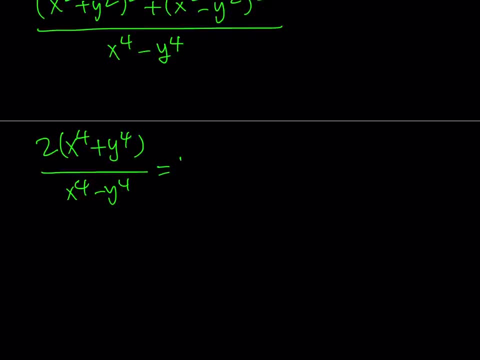 what this gives us. So this is equal to. this is equal to k, right, Okay? So from here let's go ahead and isolate x to the fourth plus y to the fourth, divided by x to the fourth minus y to the fourth. So that's going to equal k over two. So at this point I'd like to do the following. 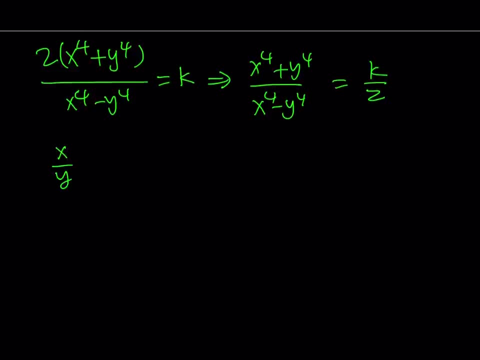 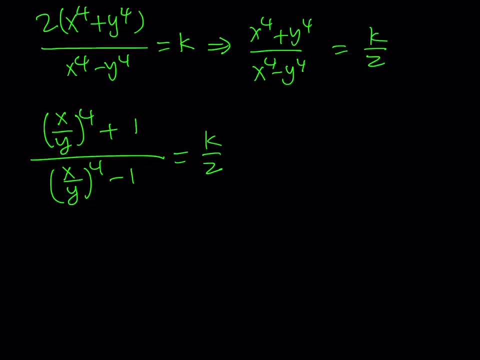 Divide everything by y to the fourth. So it looks like this: x over y to the fourth power plus one. divided by x over y to the fourth power Minus one equals k over two. So here we would like to get the x over y to the fourth power by: 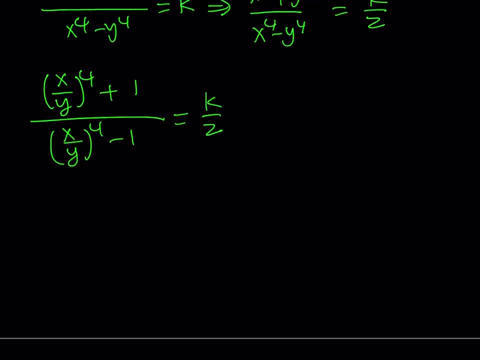 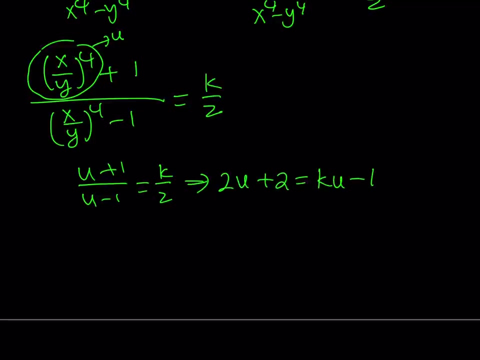 itself. So we can just go ahead and do the following: Let's just call this u, And we get u plus one. divided by u minus one equals k over two. Let's go ahead and isolate u from here: We get two. u plus two equals ku minus k. Our goal is to get u, So let's put. 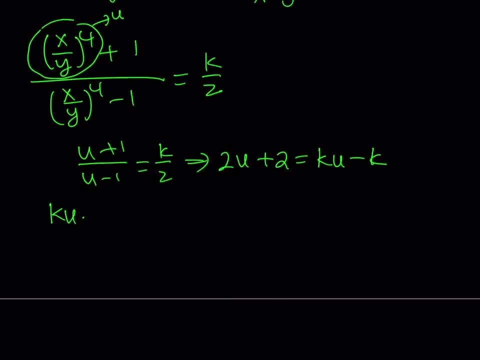 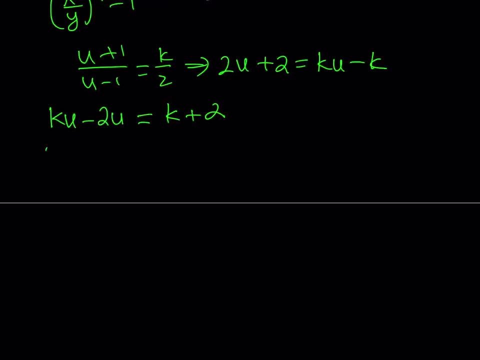 everything that has u in it on the same line. So let's go ahead and isolate u from here. Remember that song: happy birthday to you. So here we can take out the k, I mean the u- u times the quantity k minus two equals k plus two. And from here we get u equals k plus two. 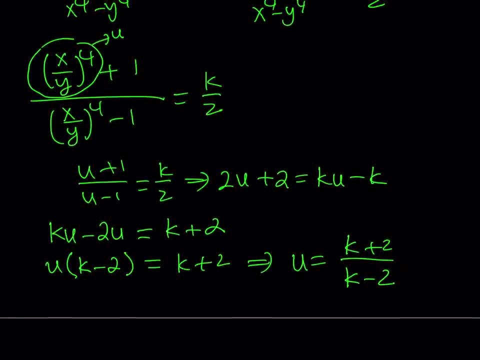 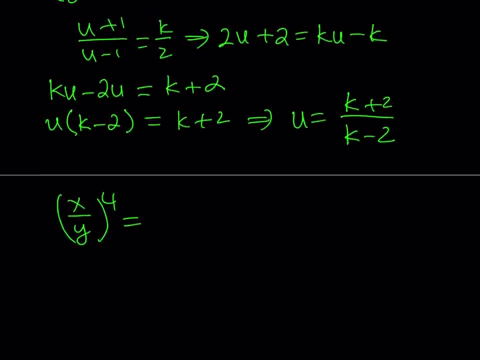 divided by k minus two. So now let's go ahead and back substitute. Remember u was x over y to the fourth power, And that is given as k plus two divided by k minus two. So now let's go ahead and back substitute. Remember u was x over y to the fourth power, And that is given as k plus two. 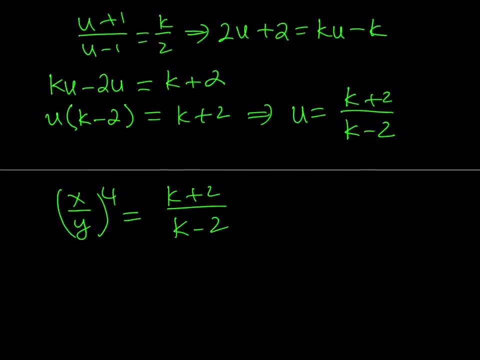 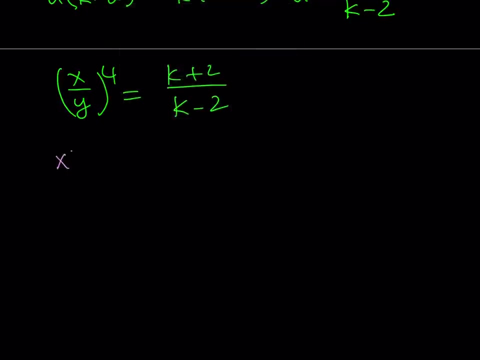 divided by k minus two, And, as you know, k is the expression given, So it's perfectly fine to write it that way. Okay, so we got x over y to the fourth power. Now let's go back to our expression. We are supposed to evaluate x to the eighth plus y to the eighth, divided by x to the. 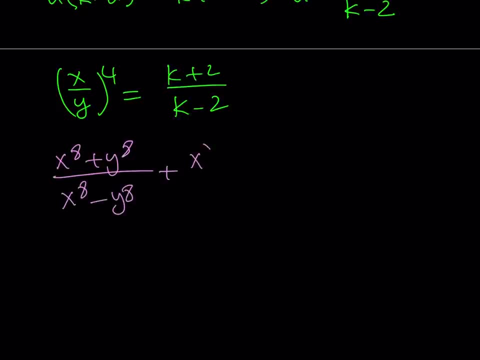 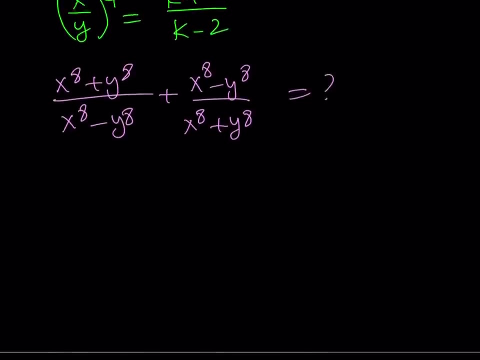 eighth minus y to the eighth plus its reciprocal Same thing, but just reversed or flipped, whatever you want to call that. So we are supposed to find this in terms of k. Now one of the things that would be real helpful is: 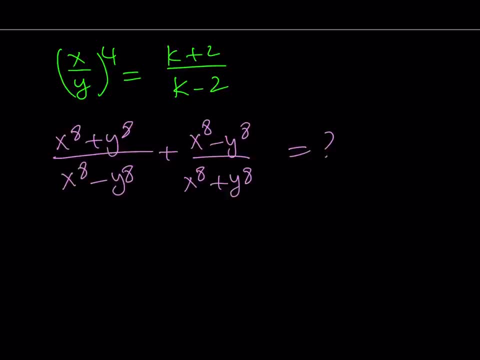 you know, follow the same method: make a common denominator. Let's go ahead and do that, And that's going to give me x to the eighth plus y to the eighth squared, plus x to the eighth minus y to the eighth squared, divided by the difference of two squares, gives me x to the 16 minus y to the 16.. 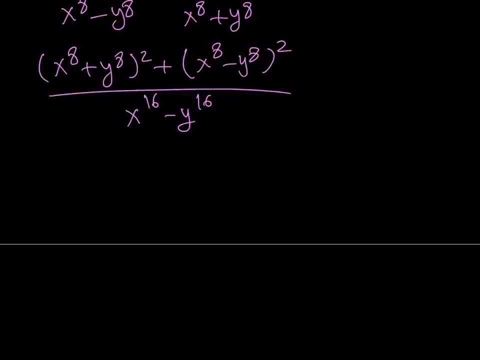 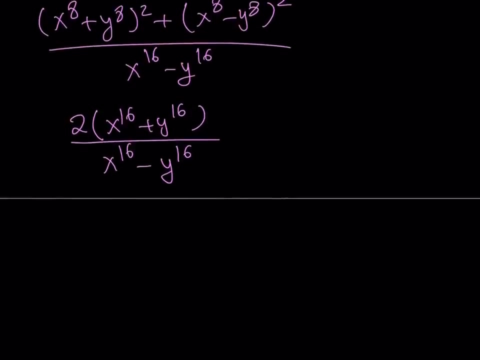 Now here we get the same identity. So that gives us two times x to the power 16, plus y to the power 16, divided by x to the power 16, minus y to the power 16.. And here we are supposed to find this in terms of k. So let's go ahead and remember what our expression. 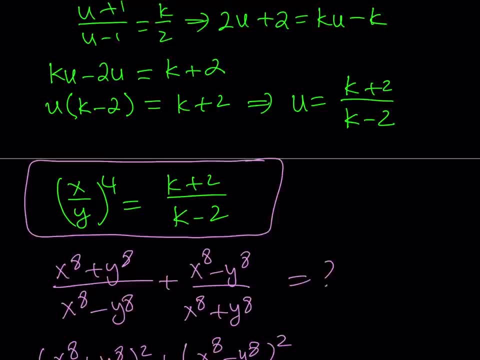 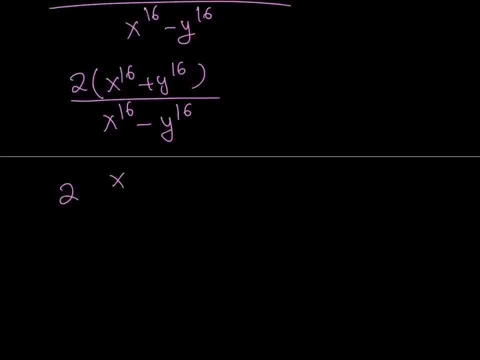 gave us the first one, we got x over y to the fourth power in terms of k. So if you can find something like that from here, that will be nice, And what I can do is divide everything by y to the 16 power. So we can get something like this: x over y to the 16 power, minus one divided by x over y. 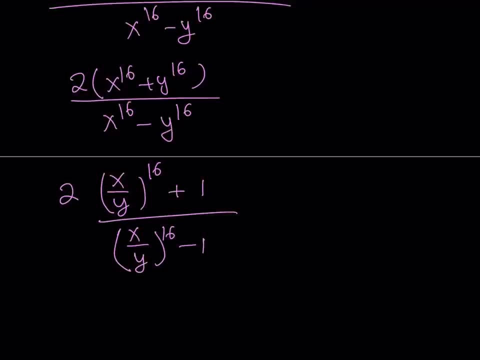 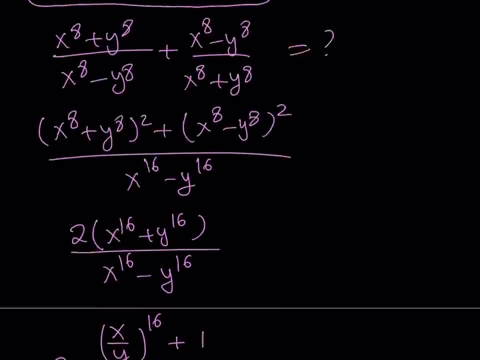 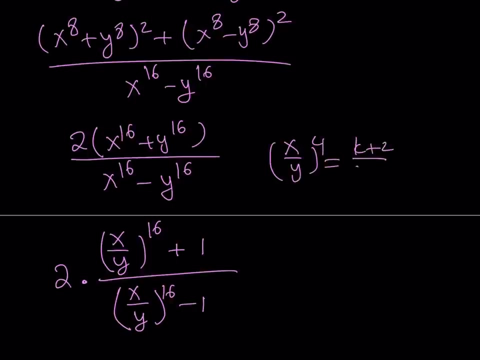 to the 16: power minus one. this should actually be a plus sign, And I can just go ahead and put the two here as a coefficient. Okay, so we're supposed to write this in terms of k, But remember, x over y to the fourth power is given as k plus two over k minus two, And now we can write this expression as: 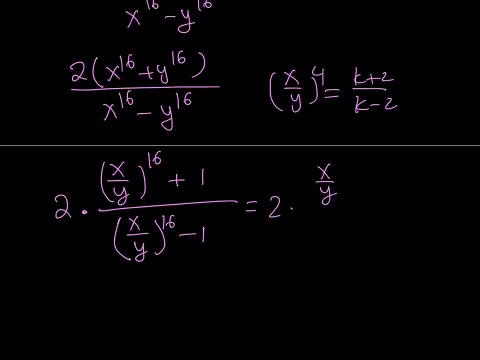 2 times x over y to the 4th power, to the 4th power. So that's going to give us, that's going to give us, basically, this expression to the 4th power, because we were raising it to the 16th power. 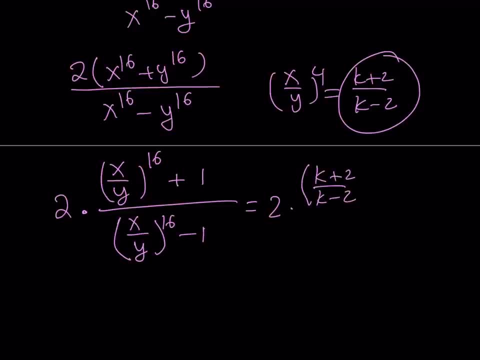 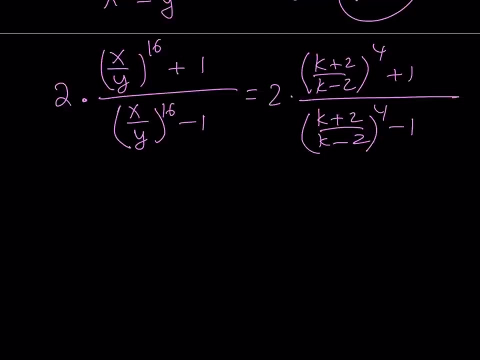 It's going to be k plus 2 over k minus 2 to the 4th, power plus 1, divided by pretty much the same thing with a minus sign. Okay, Now let's go ahead and simplify this by expanding this. We'll always have a 2, obviously, here, but we'll also make a common denominator. 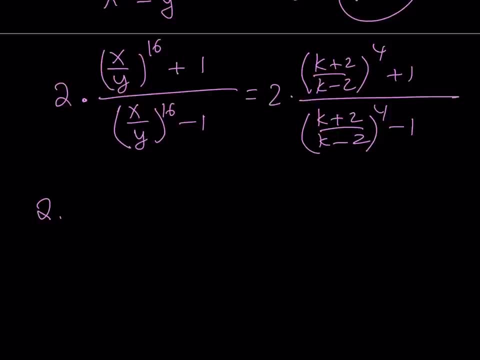 And the common denominator. actually, we're going to have two fractions that are divided, that have the same denominator, so we can totally ignore the denominators. In other words, this is what I'm trying to say. Maybe I shouldn't skip too many steps. 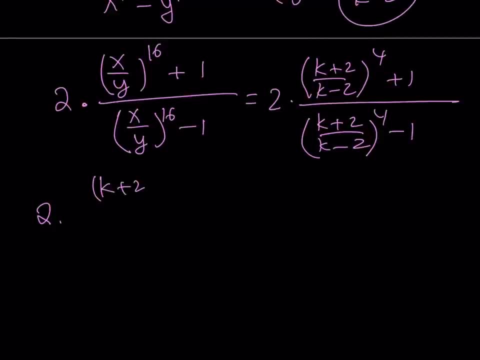 So here's what I'm trying to say. This gives us k plus 2 to the 4th power, plus k minus 2 to the 4th power, divided by k minus 2 to the 4th power. And that is all divided by k plus 2 to the 4th power, minus k minus 2 to the 4th power. 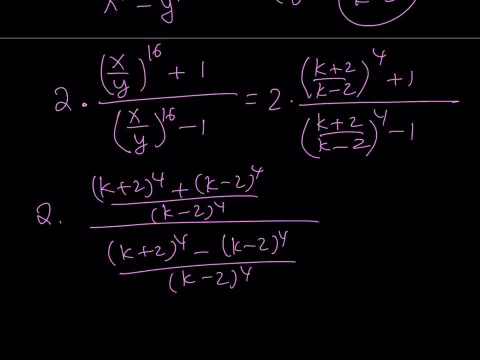 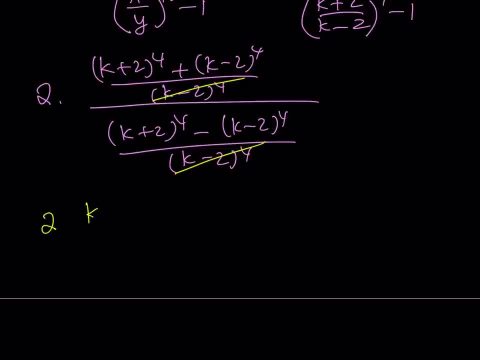 I'm making a common denominator for both fractions, And now here the denominators cancel out. That's what I was trying to say. And this gives us the following: 2 times the quantity k plus 2 to the 4th power, plus k minus 2 to the 4th power. 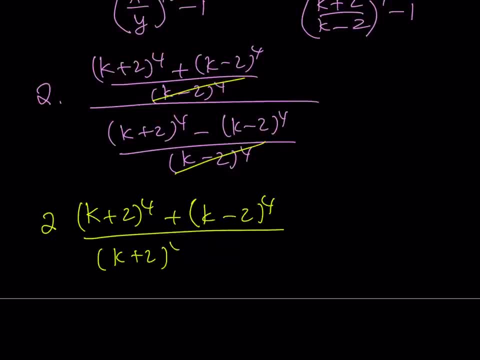 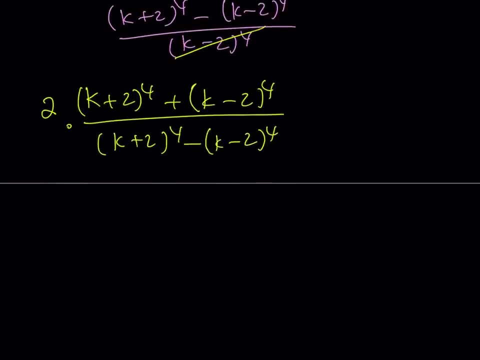 divided by k plus 2 to the 4th power, minus k minus 2 to the 4th power. So this answer is actually acceptable for the test. but I know some people are going to be upset if I don't simplify this. 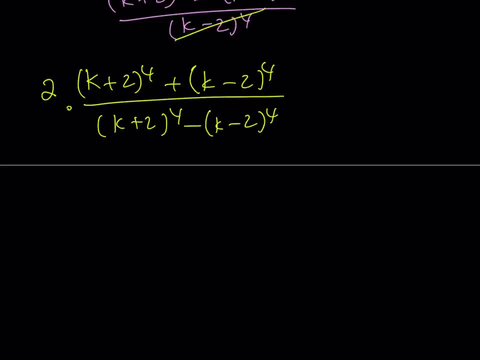 so I'm going to go ahead and simplify this expression and give you the result in the final, I mean in the simplest form, in a way. So this is multiplied by 2, and if you go ahead and expand this from binomial theorem: 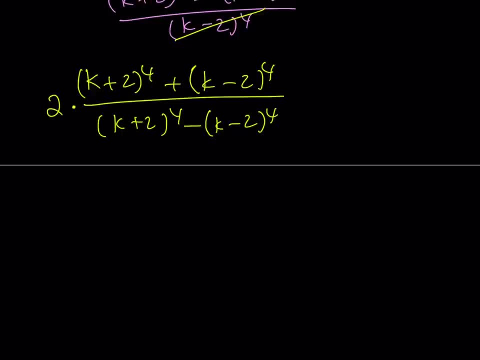 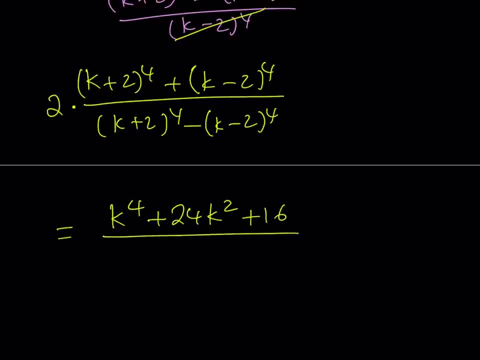